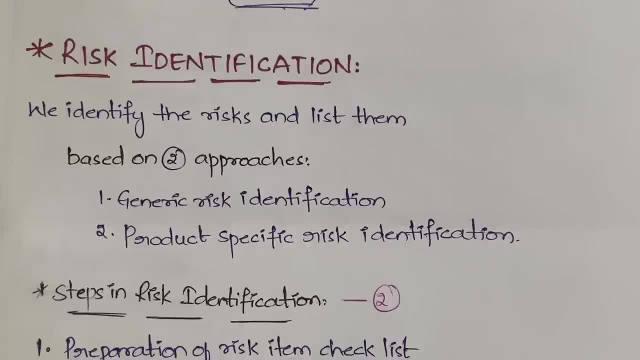 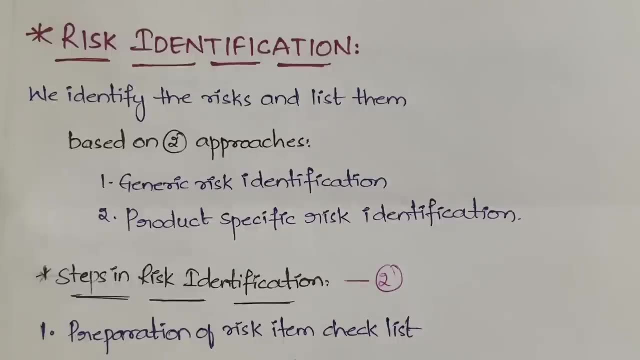 writing it in such a way that you can understand it clearly in a simple English. I'm writing, So in some situations I will have to just read out what I've written, So I'll try to explain it, But still okay. So yeah, first is risk identification. Here, in this identification step, what we do is it is not like step by step, risk identification, then risk, you know, projection, refinement. it is not like all these are activities So we can do them in any order. So first we will identify the risk. 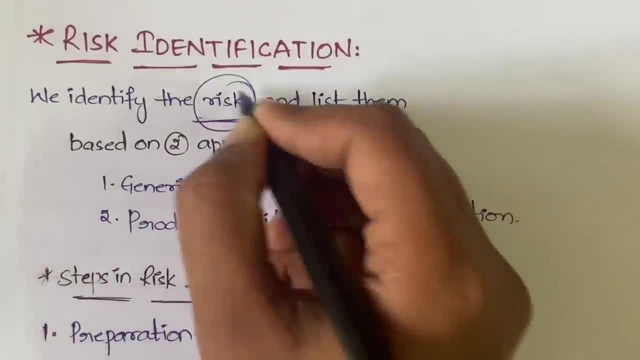 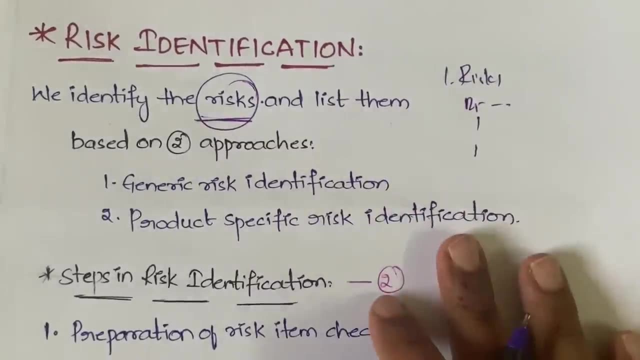 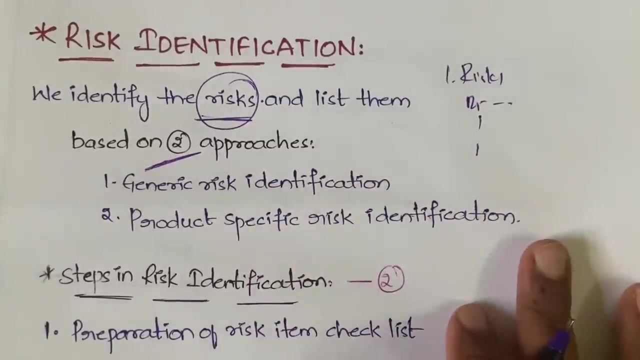 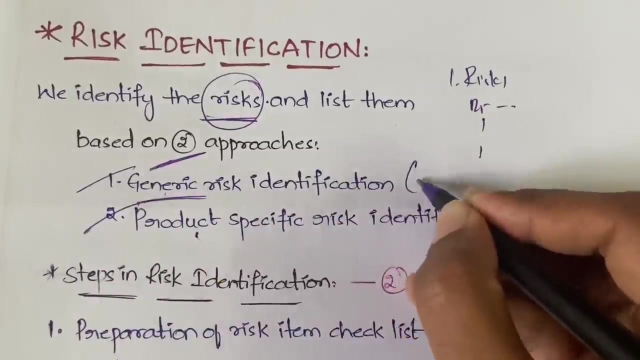 and list them. So we will identify what are the possible risk and make a list of them. That is risk one, risk two, like that. we make a list of all the risks. Got it So here, actually, while doing the risk identification, we have we have two approaches, that is, we can follow any one of the approach. First is a generic risk identification. Next is product specific risk identification means what I'll tell you. generic is nothing, but in general, or you can say overall: Okay, so not in a particular area, suppose in your 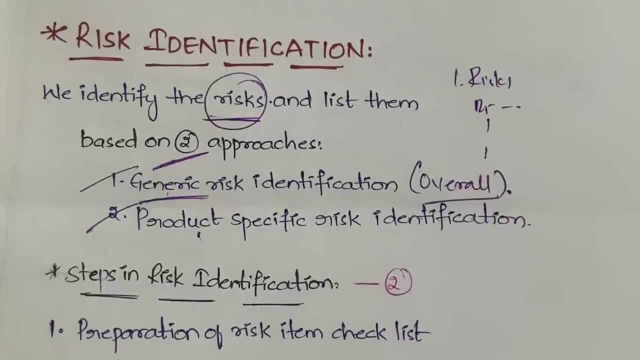 house. we have different rooms, right, We have living room, we have the main drawing room, bedrooms, kitchens- sorry, kitchen washrooms and all So you are cleaning the entire house. that is overall house you're doing. So that is generic. product specific is okay. today we don't have much time, So for now, let's. for today, let's clean only bedrooms, Or for today, let's, you know, start out only bedrooms. If you're doing in that way, that is only particular things you're doing. That is product specific: risk identification. In generic you. 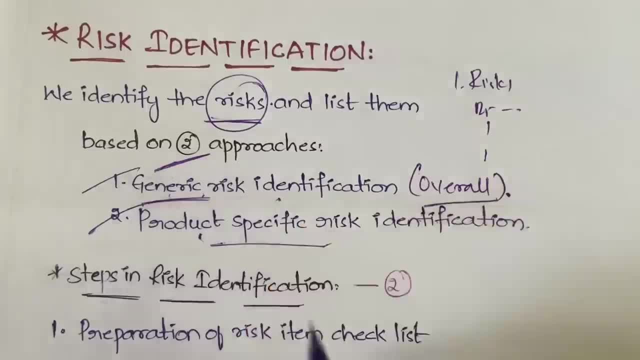 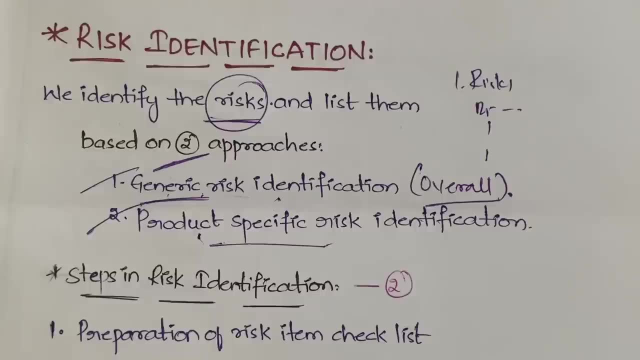 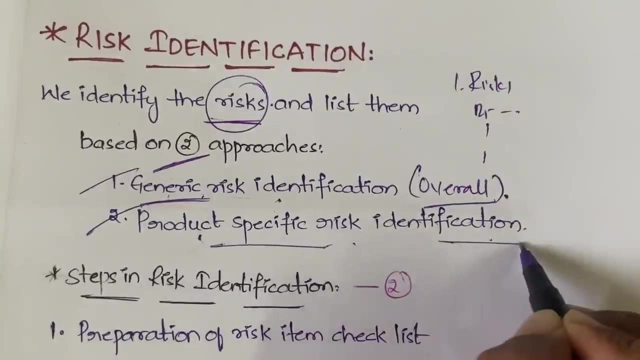 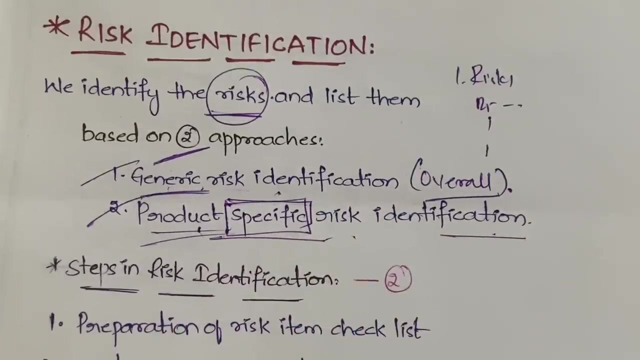 will be concentrating on overall status. In generic risk identification, you will be concentrating on the entire software. you will be concentrating on the entire organization or entire application. you will be concentrating and you will be taking out the risks. But in product specific risk identification approach, what you will do is those are specific to the particular product. you will be doing it. Got it Simple. Now let us see what are the steps we have in risk identification. See, actually we have only two. 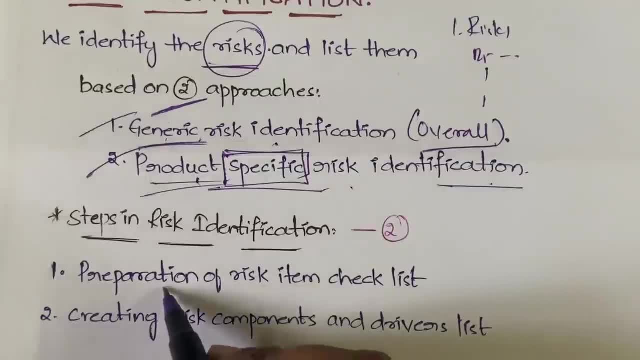 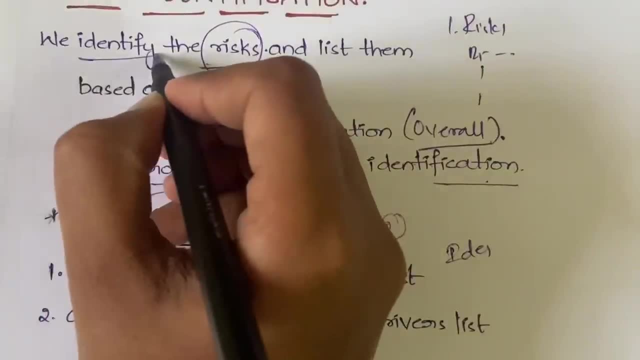 steps in risk identification. okay, first is preparation of risk item checklist. that is, as i already said, what you have to do. you have to first- yeah, here it is. you have to first identify the risk and prepare a list. right, you need to prepare a checklist. you know what is a checklist? 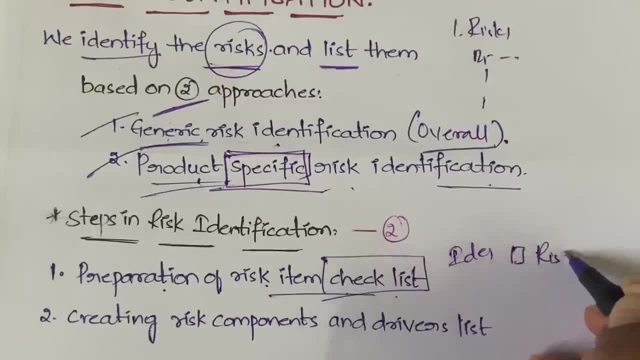 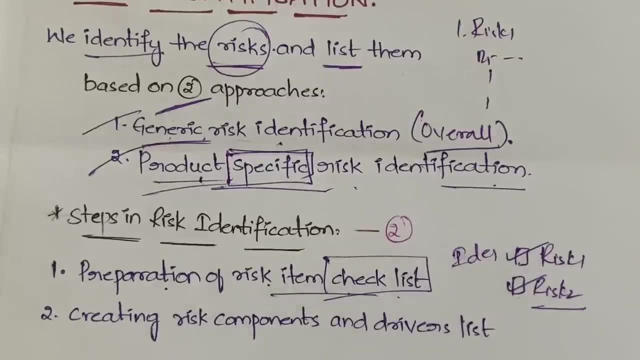 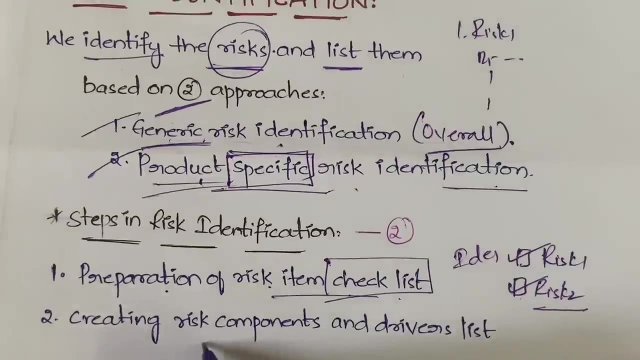 right. you will have a box and risk one box, risk two. so if this is cleared, this will be checked. if risk two is cleared, this will be checked. so you need to prepare a checklist first. okay, once create. after creating the checklist, you have to create the risk components and drivers list. 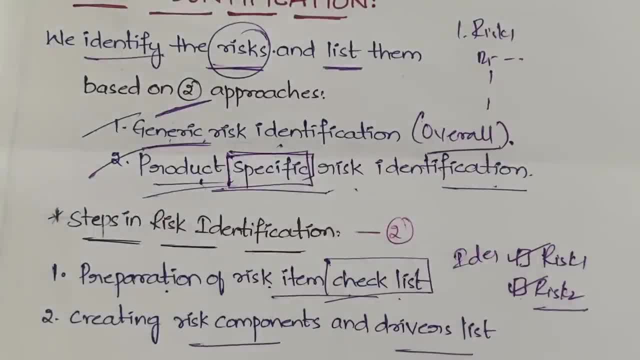 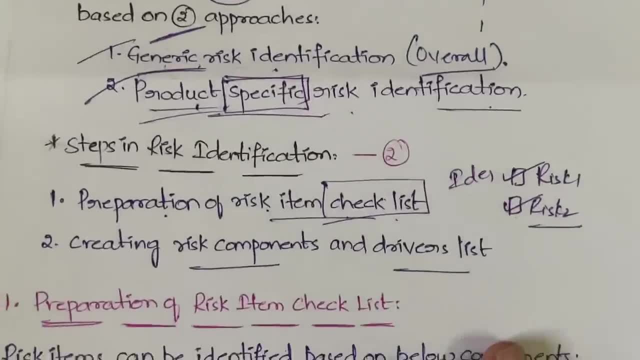 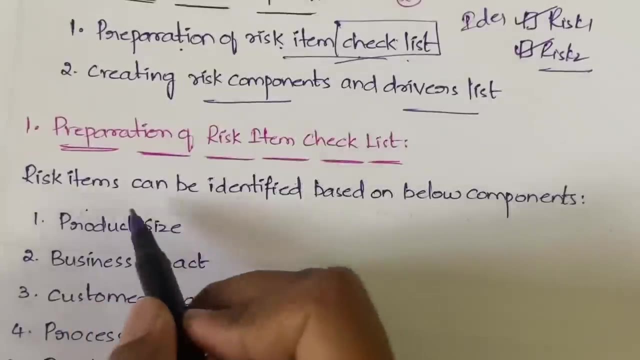 okay, so what you have to do in this components and drivers list, all i'll tell you, don't worry. so in that, let us see about each step in detail. now what is the first step? preparation of risk items checklist. right, so in the preparation of risk item checklist, risk items can be identified. 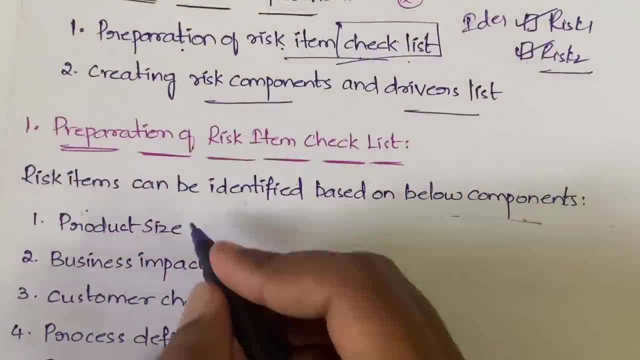 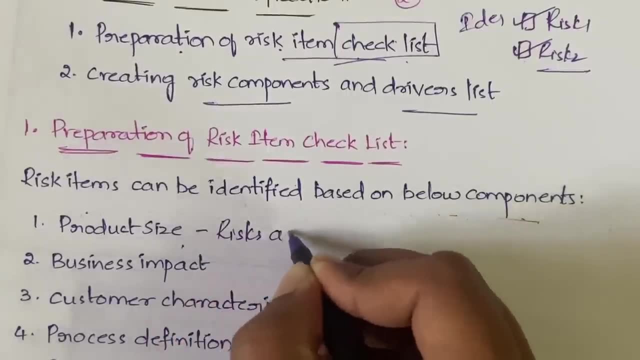 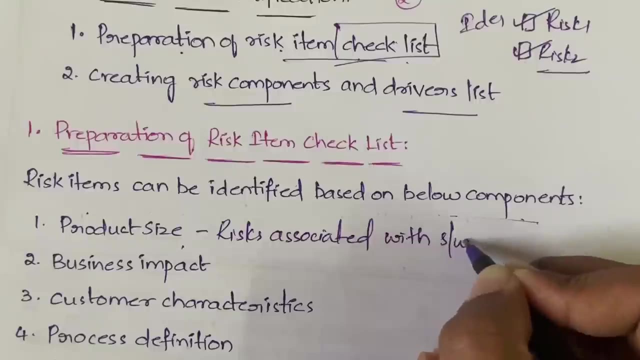 based on below components. okay, so first one: product sites. what do you mean by product sites? so in the preparation of risk item checklist, risk items can be identified. product size: it is nothing but the risks which are associated with the size of the- sorry if i'm writing any spelling mistakes- with the size of the software. okay, that is a product size. next is: 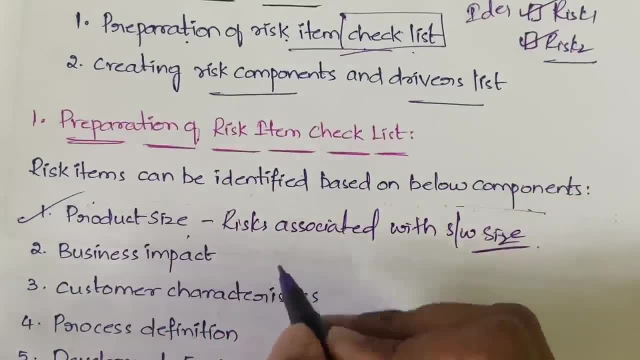 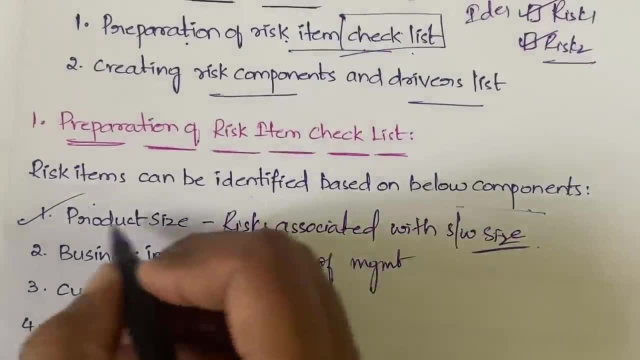 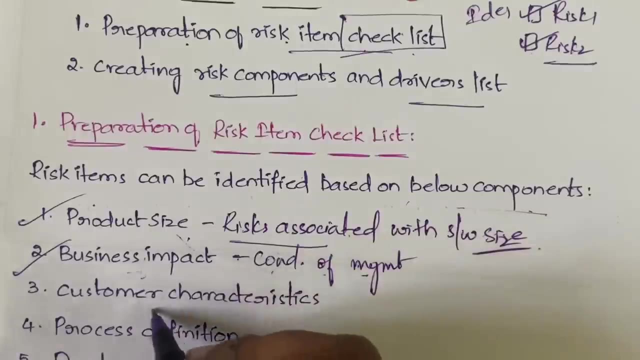 business impact. so the risks associated with the conditions which are imposed by the management, conditions of management, the risks which are occurring or the risks which are associated because of the conditions which are imposed by the management. okay, next comes the customer characteristics. customer characteristics it is- uh, you know, the word itself says the. 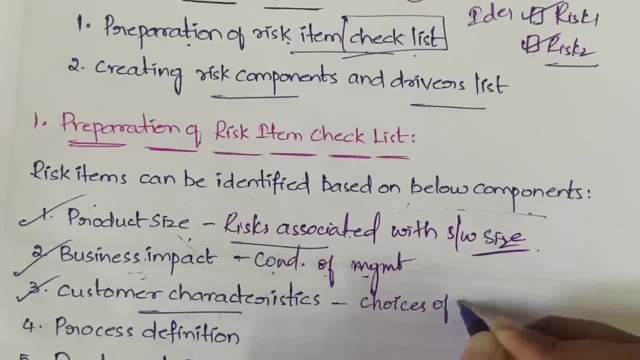 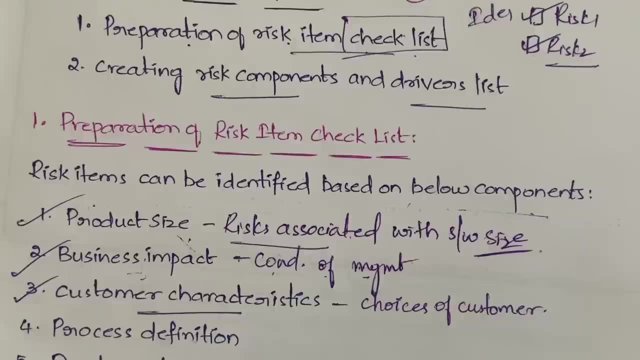 the risks which are associated with the choices of customer. okay, so each customer will have different choices, right? every per every person is not the same. everybody will have their own interest, their own choices. so, the risks which are associated with the choices of the customer, because you know you need to. 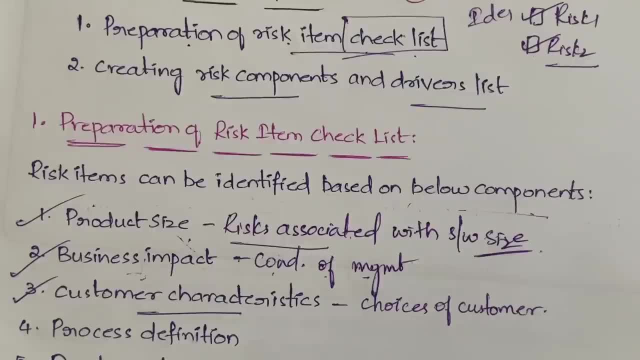 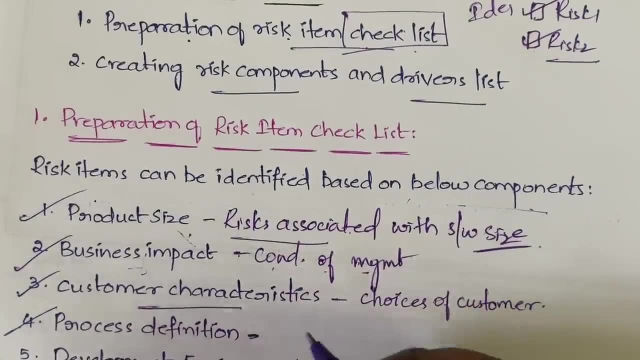 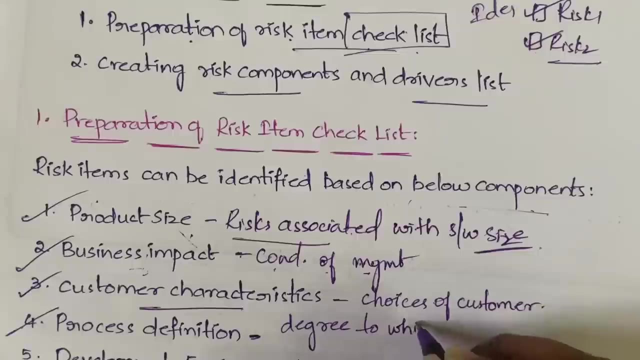 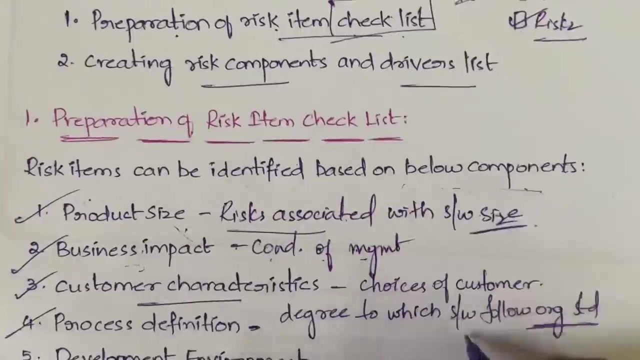 design a product in to one customer in one way, to the other another way, like that. next comes the process definition. process definition is nothing but the risks associated with the degree to which software will follow the organization standard. okay, the degree to which the um, you know software will follow the organization standards, that is, the organization will have some 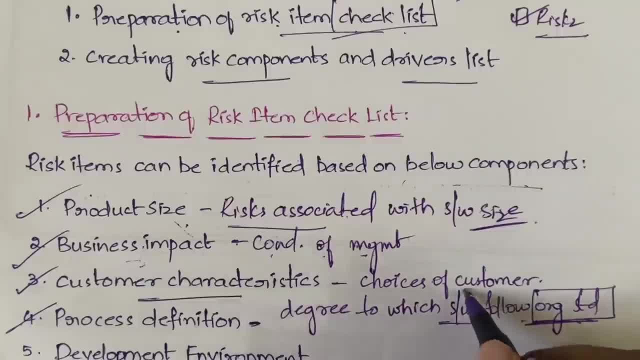 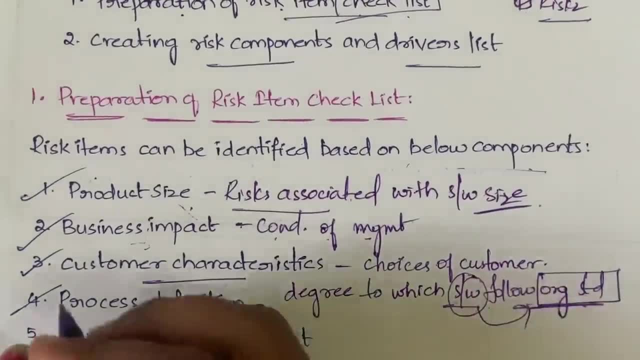 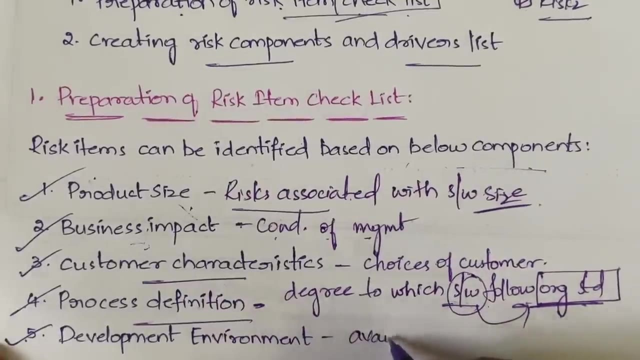 standard setup right. so up to what extent the software which we have designed is following this? if not, risks will occur. so those risks will come under the process definition. okay. the fifth is development, environment, development. one environment is nothing, but you know the risks associated with the availability of the development tools. you can say availability of development. 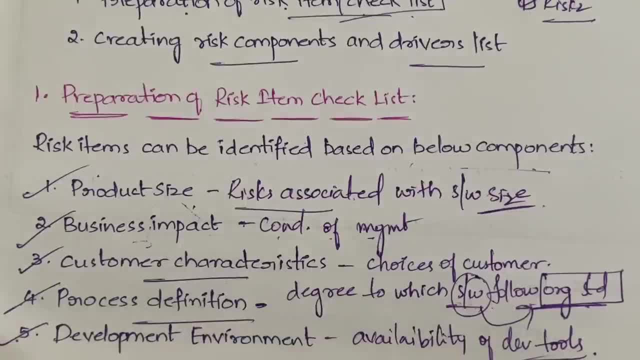 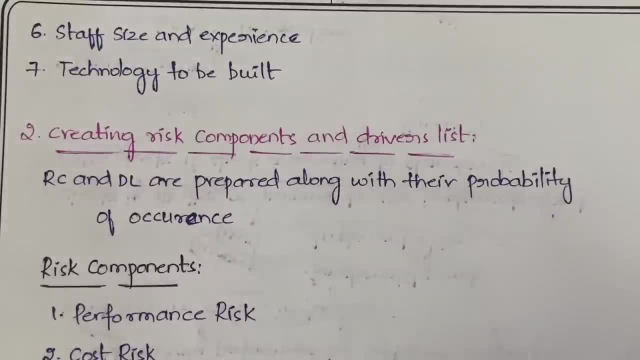 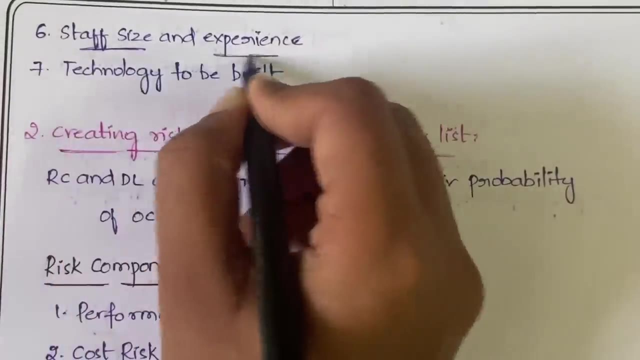 tools got it. the risks which are associated with the availability of development tools or development environment, those will come under the development environment category. the next category is taps size and experience. staff size and experience if the it itself says how, how many, how many people you have in your organization and what is the experience they have, that is, if all. 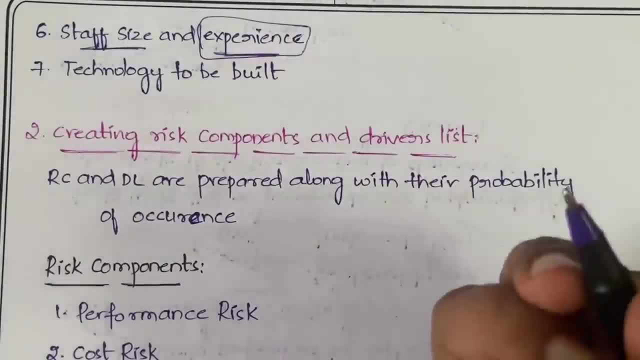 our freshers, then it is a problem. right, because any problem will occur, or if any, they don't know anything. pressures- usually they don't know anything. they have to be given training first and all, and also technology to be built. if there is any research related issues, most of them are not given training required. the accuracy of the work done is not за relevant, and all the tips and things required for it are sometimes not surely lash. okay, first and foremost, try to maintain integrity. so the 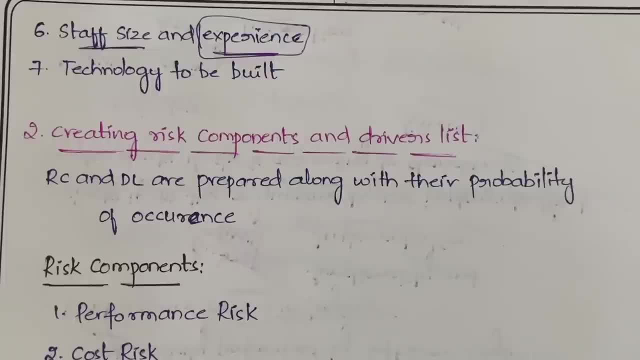 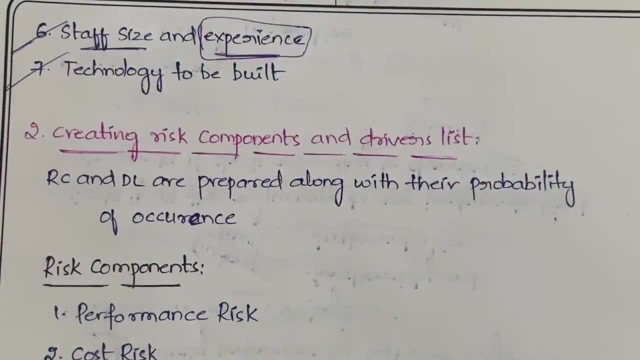 risks associated with the technology on which we are, you know, generating that software, creating that software, then, in that case also. so, based on all these things we need to create, we have to consider all these things and we need to prepare a risks checklist. got it now, after creating the. 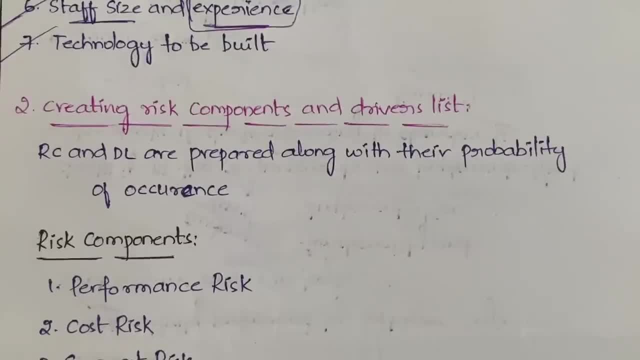 checklist, you need to create the risk components and the drivers list right? so rc is nothing but the risk risk components and deal nothing but drivers list. so in preparing the risk components and drivers list, you need to do it with the probability as well. that is the probability. 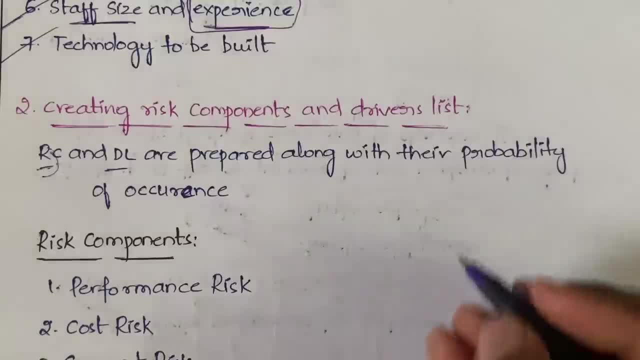 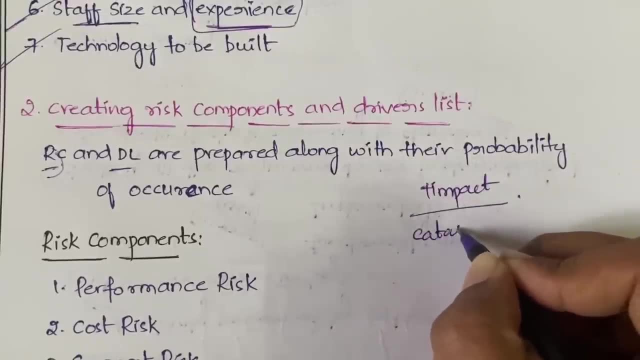 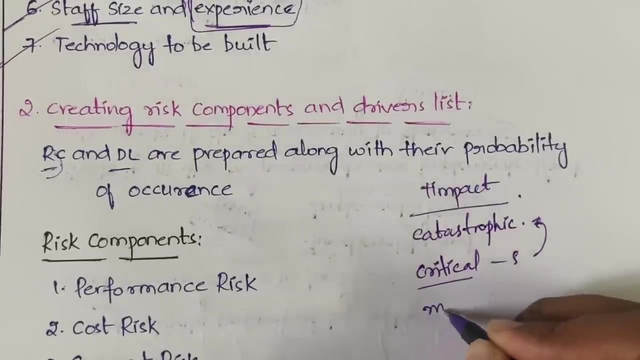 of their occurrence. right, that is, you need to additionally add the impact, that is, that impact could be catastrophic or catastrophic, whatever you call it. that is critical. next one, I'll tell you: catastrophic. so critical means you know it is very serious. so catastrophic is more, it is more dangerous than critical. okay, next is marginal. 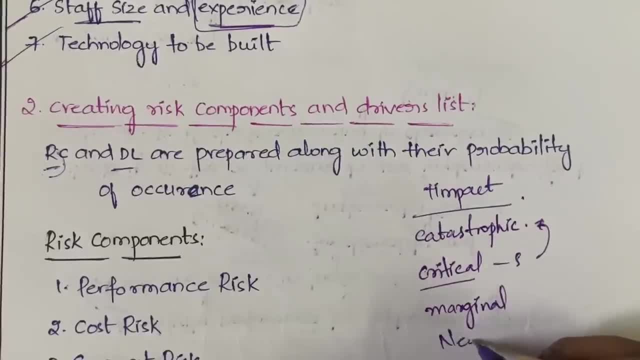 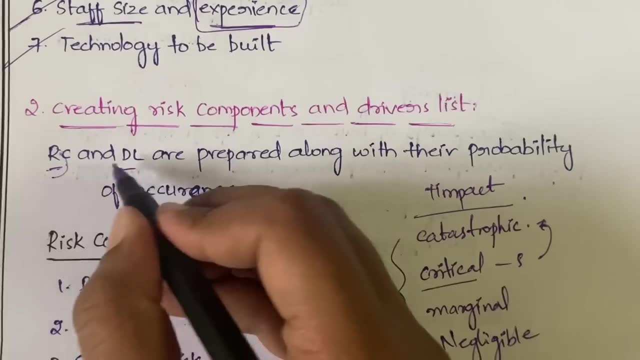 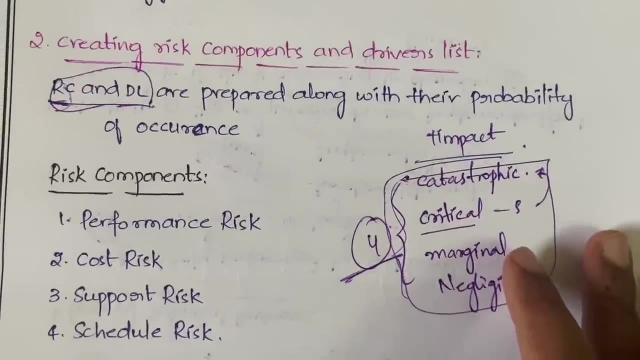 next is negligible. okay, you will have total four impact categories. so when you are creating the risk components, and the drivers list along with their impact category also has to be included. okay, so how many types of risk components we have is we have four types of risk components and that the 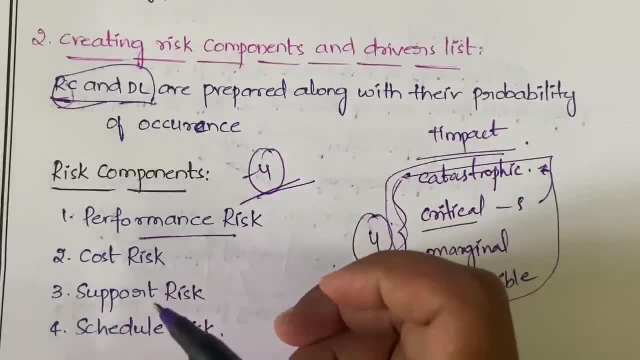 first one is the performance component and the second one is the risk component and the third one is the performance risk. that is, for what purpose we have created it. we have created the software for what purpose. we have produced the software for what purpose and whether it is serving that or 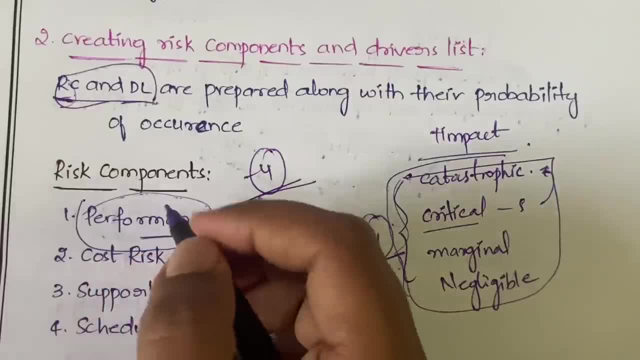 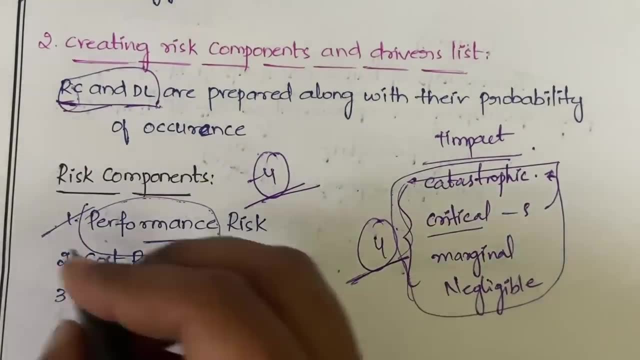 not the whether the performance of software is good or not. if not because of the performance of the software, whatever risks are arising, those will come under performance risk. cost risk again, if the budget is maintained or not. if the budget is not maintained, then cost risk will occur next. 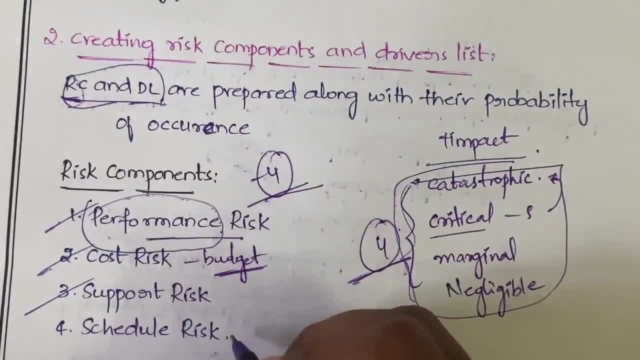 is support risk. so what do you mean by support risk? uh, you know, you know what is support after you deploy it to the client. after you deploy a software to the client, you have to maintain the software right. so in maintenance you will be doing some support activities, like if there is any issue. 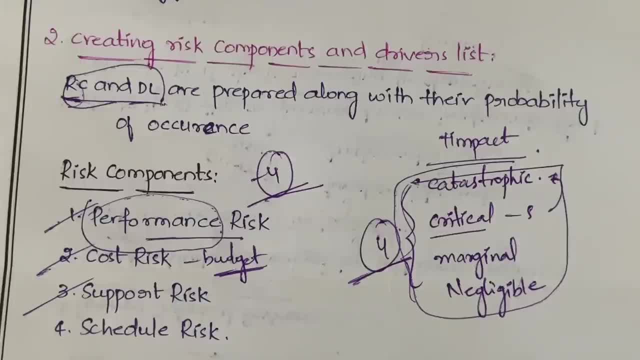 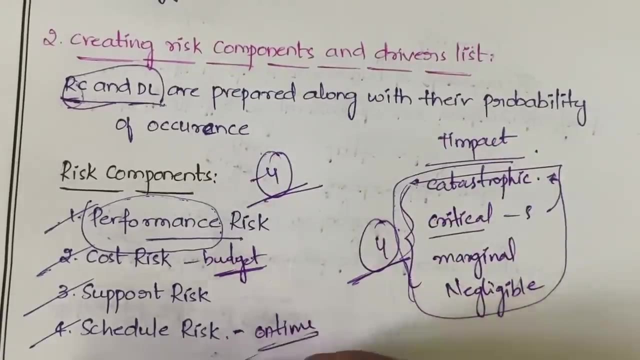 like, if there is any a problem if they are not, if the client is not able to access any website or any module of the website or application, and also support activities. you know that. so the risks associated with the support activities and schedule risk. schedule risk is that whatever the client has asked or the customer has asked, whether you are able to do it on time or 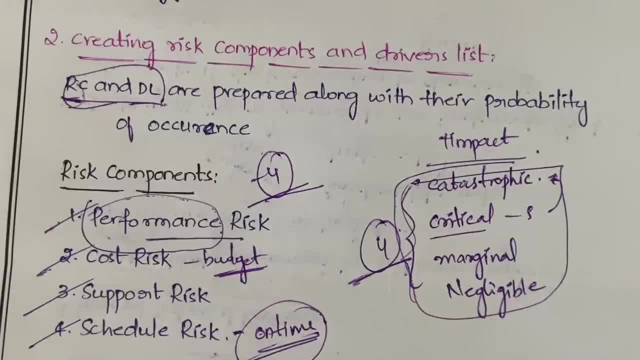 not see client or customer. anything refers to same. since I am, you know, habituated to the word client in the office, I'm using client more. okay, don't mind client or customer, anything is same. so schedule risk is nothing. but whatever customer has asked whether we are able to do it on time. 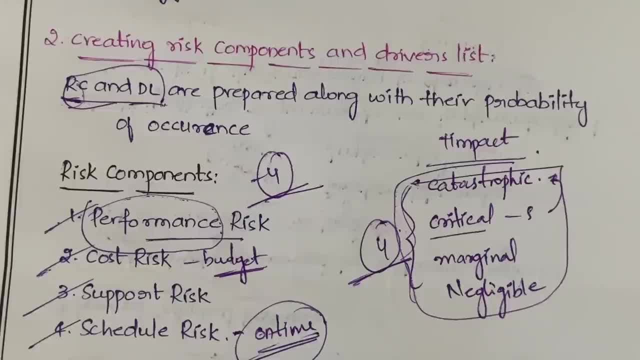 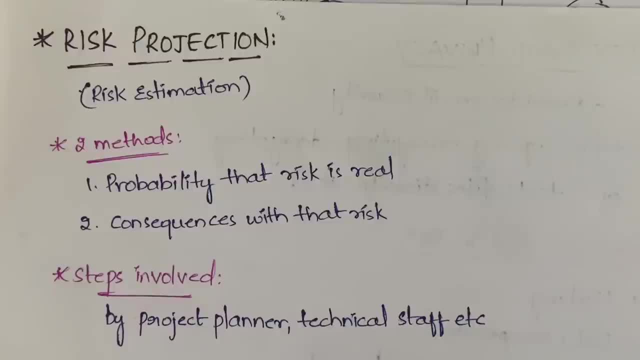 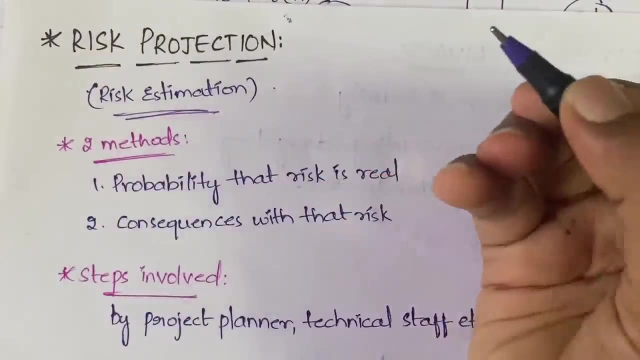 or not got it? so this is about the risk identification. next, risk projection and risk requirement. are not these this long? okay, after risk identification we have risk projection, then risk refinement, then rmm. so in risk projection it is also called as risk estimation. here you, simply you will estimate the risk. got it so here? 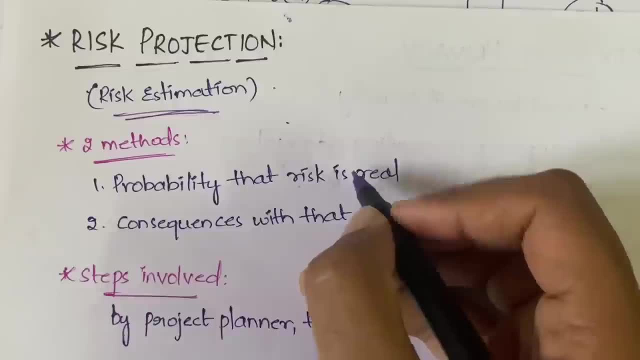 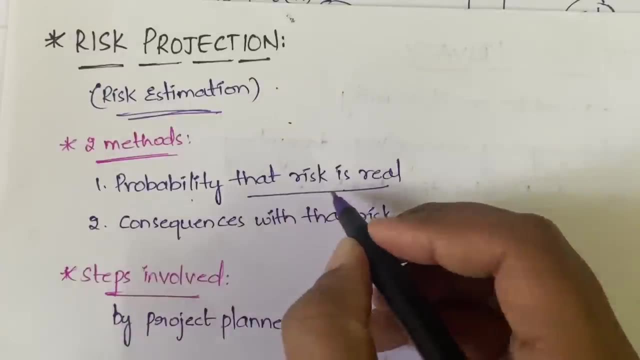 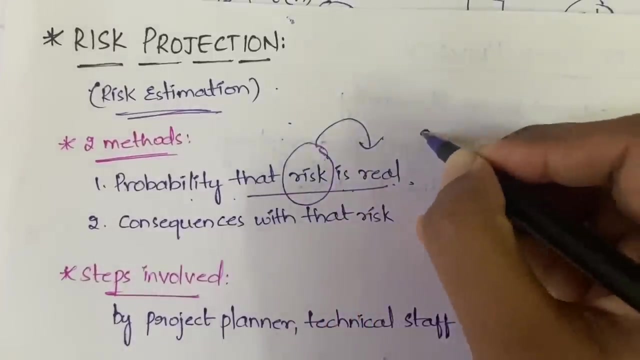 also, we have again two strategies or two methods you can say so. the first one is probability that the risk is real. that is, you can do the risk estimation by assuming that the probability that the risk is real. so what is the probability that the risk could become reality, whether it is. 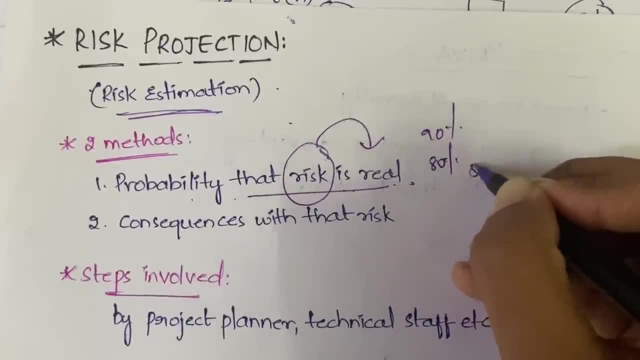 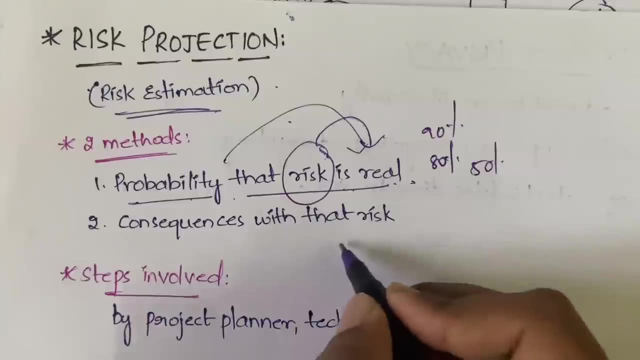 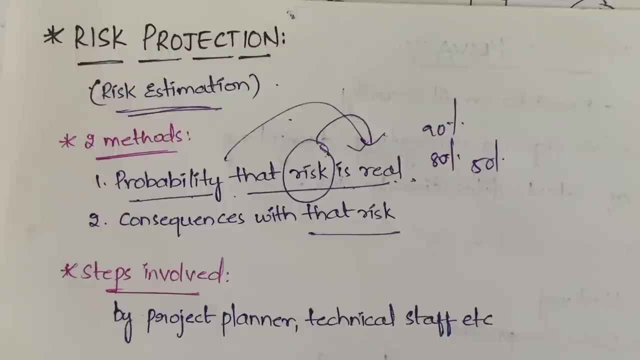 80 percent, or whether it is 80 percent or whether it is 50 percent. so what is the probability that the risk could become reality? based on that, you can do or consequences with that risk. if that risk happens, if that risk becomes reality, then what are the consequences that we have to face? okay, so this: 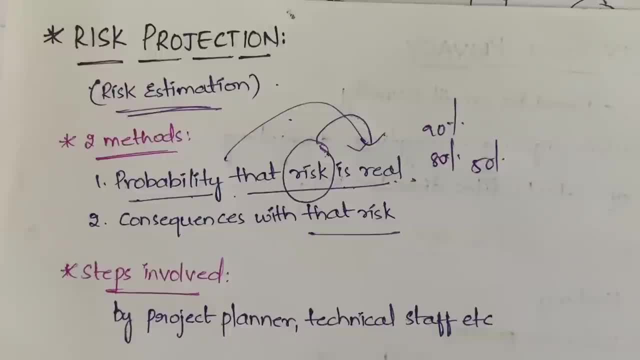 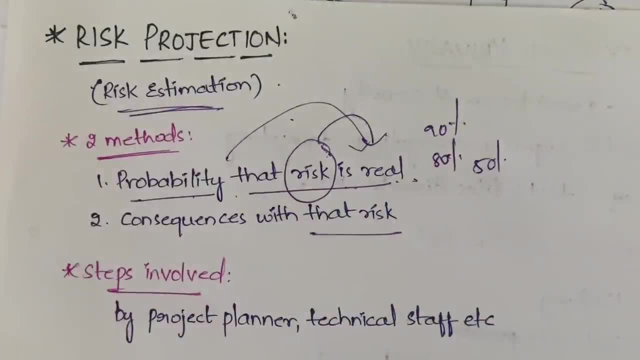 is about the methods we have in this projection. so you can do it in any of the method got it. so here in risk projection actually we have a few steps. we have around four steps. all these four steps are performed by whom? these four steps are performed by the project. 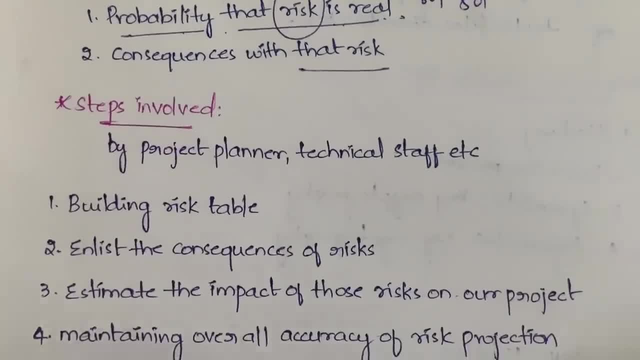 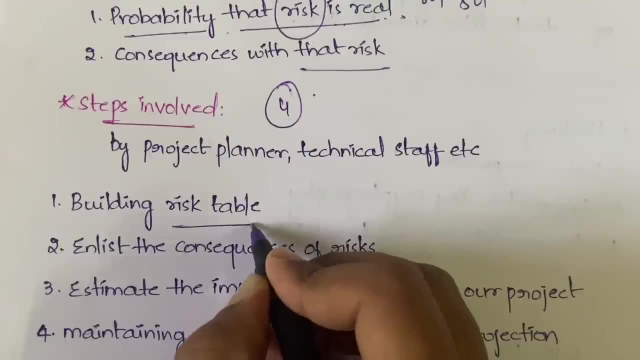 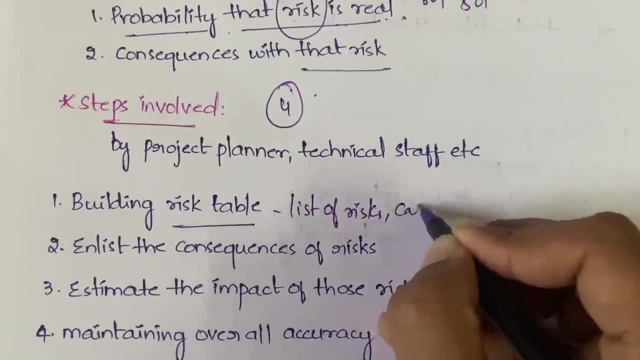 planner, the technical staff and all these people will do. okay, we have four steps here. I will tell you what are those. first, is you have to build a risk table. okay, risk table will have the list of all the risks- okay, risks- and the category, under which category they come, and also the probability. 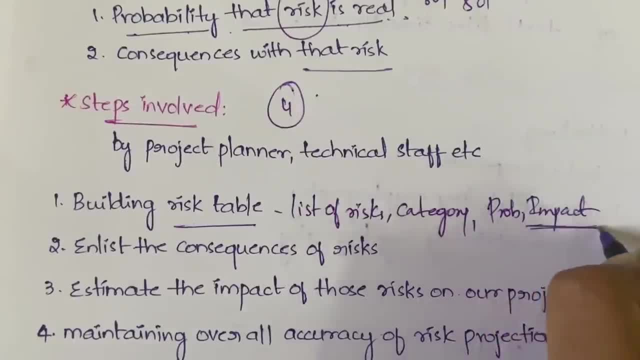 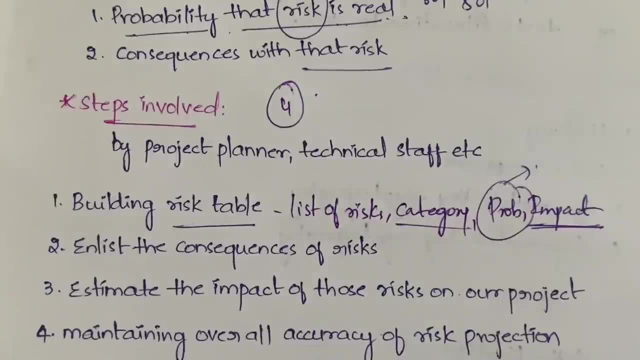 of those risk and impact that is catastrophic, critical? we have no and a probability, how, what is the probability that the risk happens? and the category- whether they come under performance risk or cost- is budget risk and we have so many types of risk right and the category of risk list. so we have to, we have to. 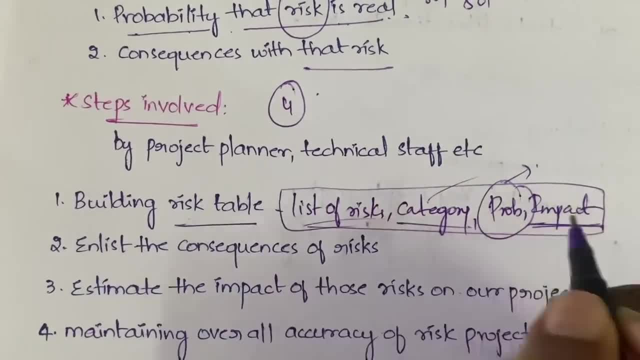 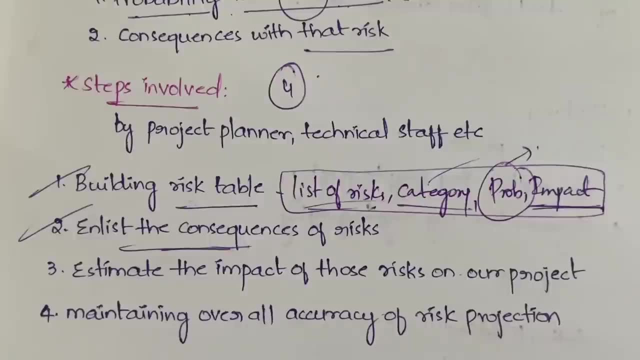 first, build a risk table by using. all these things have to be included in the risk table. in the second, what you have to do, you need to enlist the consequences. that is, if this risk happens, what are the problems that we are going to face? so you need to include all those consequences also. 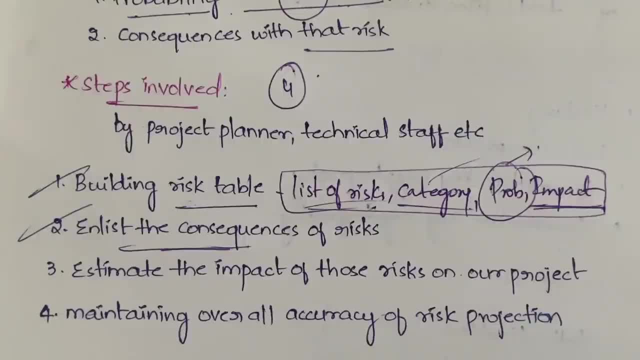 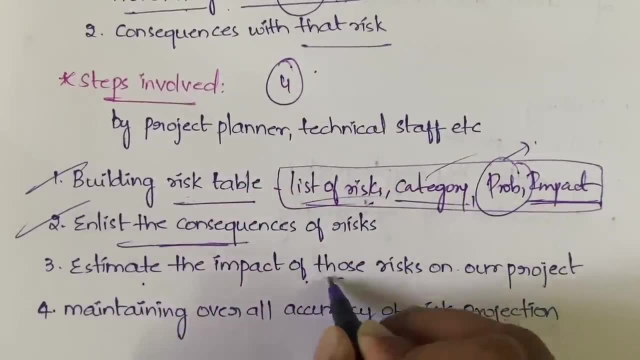 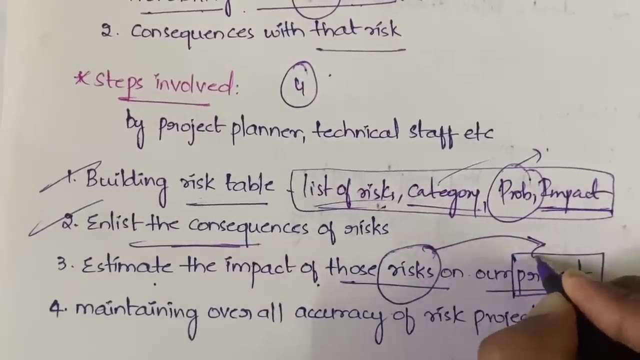 okay, you need to enlist all the consequences which are associated with each and every risk which you have mentioned here in the risk table. you got it. next, estimate the impact of those risks on our project. so, on our project, what impact these risks are going to have. that is how they. 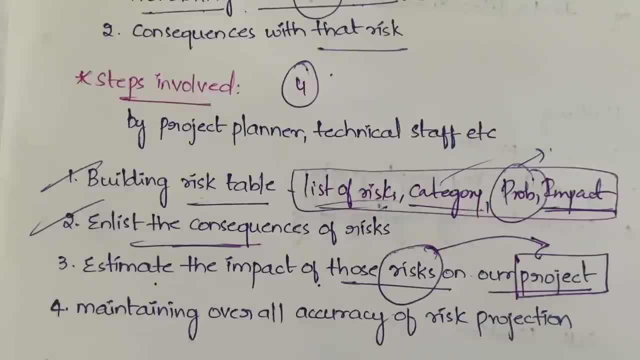 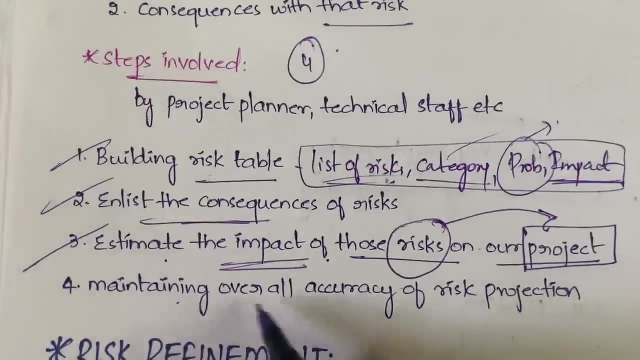 are going to modify our project. they are going to change our project in what way they are going to change our product, in what way they are going to affect our project. that we need to estimate, estimate the impact, the effect. okay, next, maintaining overall accuracy of the risk projection, the 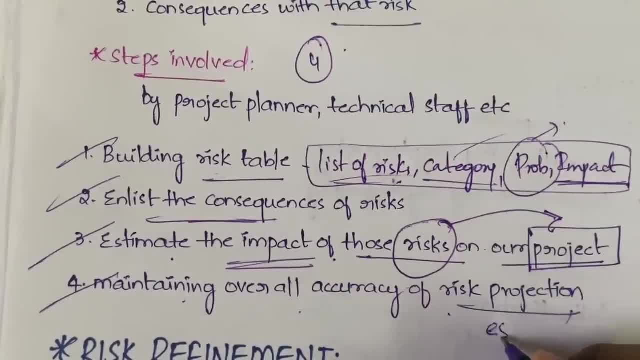 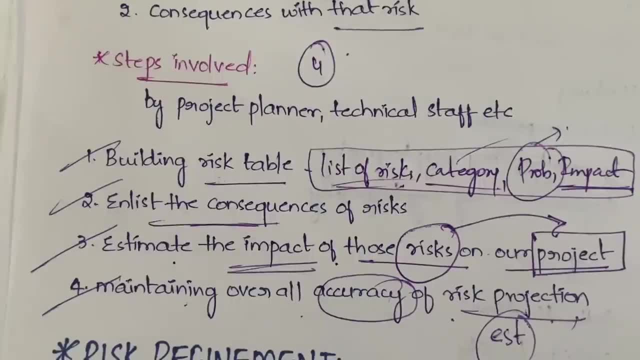 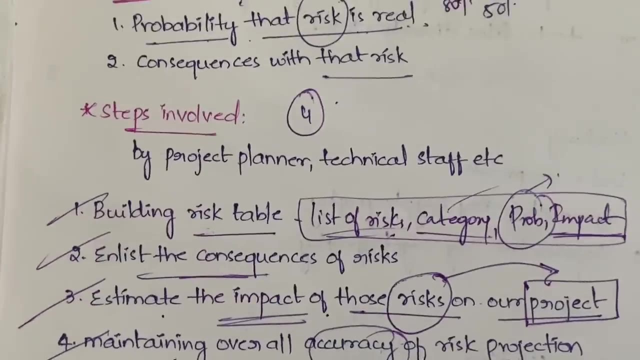 last one, that is, risk projection. that is, risk estimation has to be done accurately, because this is very important, because you are estimating the impact of the risks here. okay, so this is about the risk projection. in this you have two methods and four steps. that's all. so after risk projection: 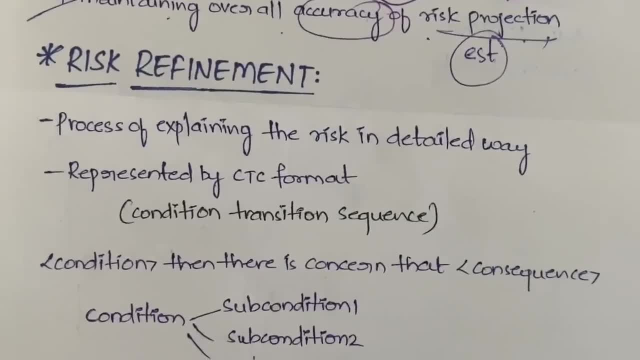 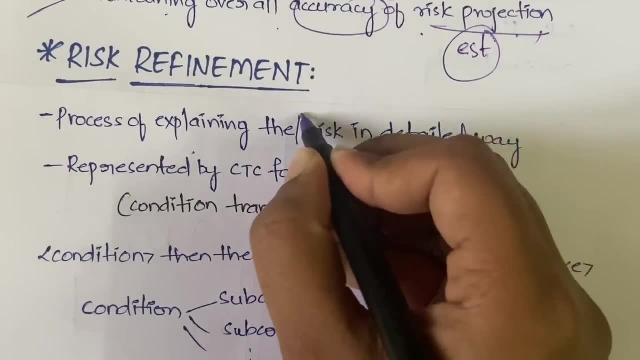 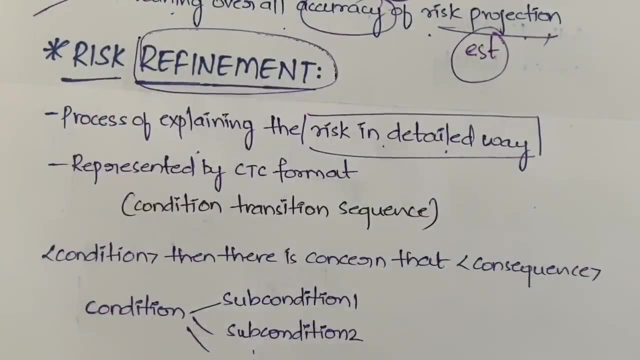 what is the next thing? we have risk. refinement again. this is also simple, don't worry. so basically it is a process of explaining the risk in a detailed way. refinement- the word refinement itself says you remove all the impurities and you get the pure matter right here also. 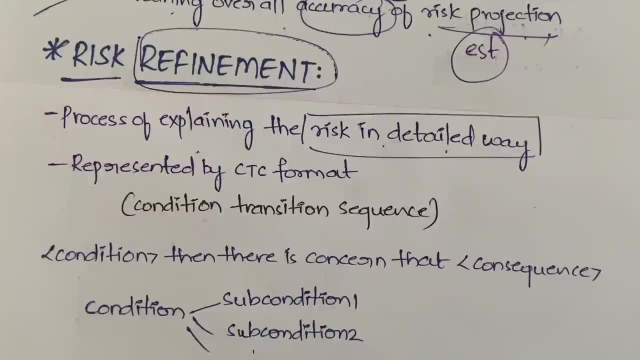 everything in detail you will get. so, whatever unwanted data is there or whatever unnecessary data is there about the risk, all that will be removed, only details about risk. that too, in a very, very depth, in depth, detailed way, will be mentioned in the risk refinement. okay, it is represented by. so actually, why here we do it in a detailed way is 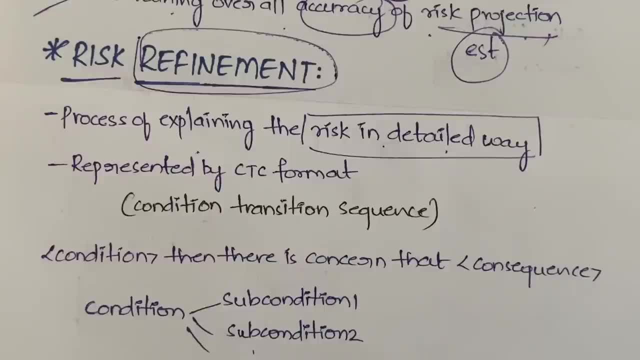 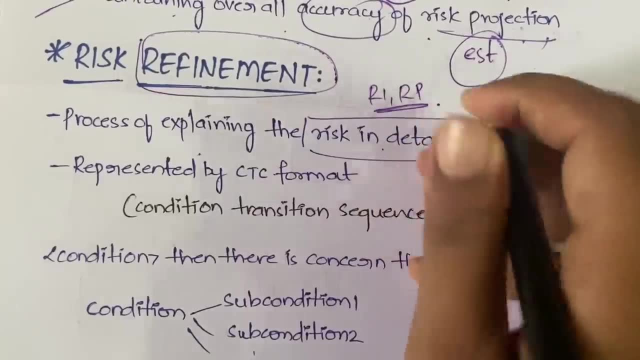 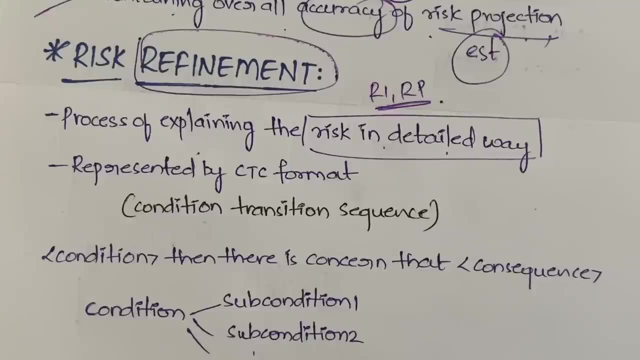 how we can get a detailed description about risk is initially, in initial stages, like risk identification or risk projection, what we are doing. we are just in risk identification, we are just identifying the risk. in risk projection, we are just estimating the risk. so we have studied about the risk already. in risk identification, we studied 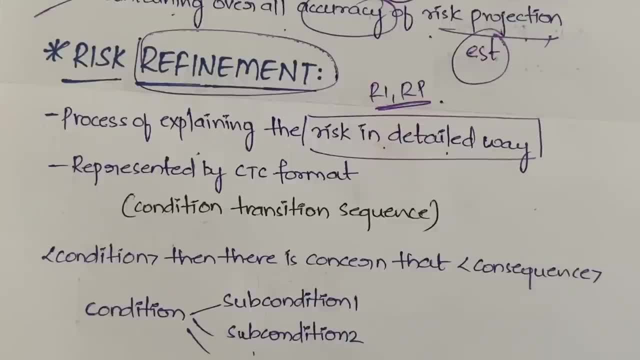 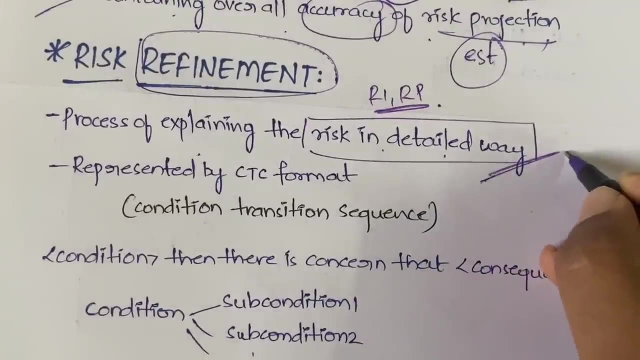 about the risk in risk projection step we studied about. so by now, by the time we reach to the risk refinement activity, we will have complete idea about the risk, because we have done a lot of work on that right. so that is the reason why here you will have a lot of knowledge about the risk. so you 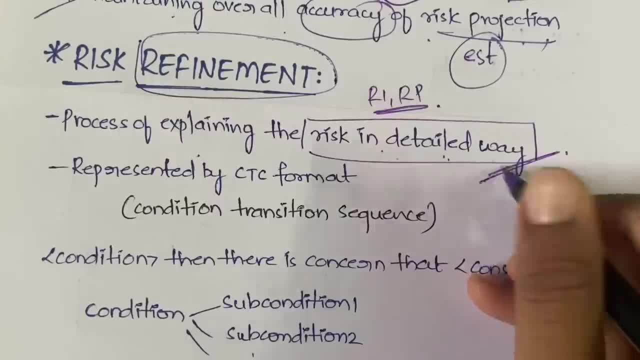 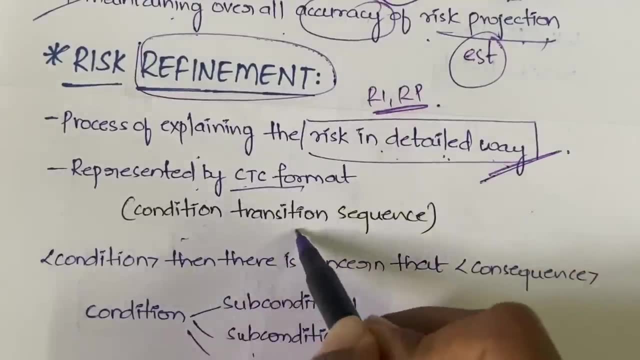 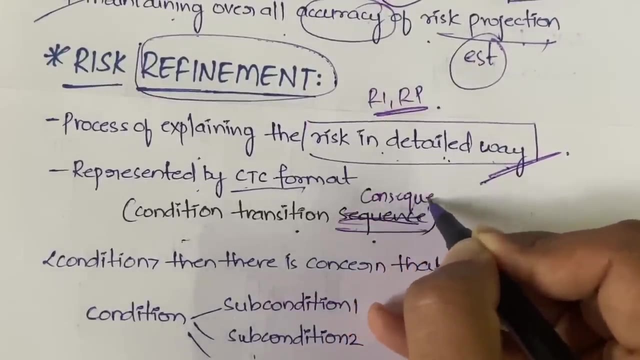 will be able to explain it in the detailed way. okay, and it is represented by CTC format. what do you mean by CTC format? condition transition sequence. sorry, it is not sequence, it is consequence. okay, condition transition, consequence. got it. so this is nothing, but you will be. 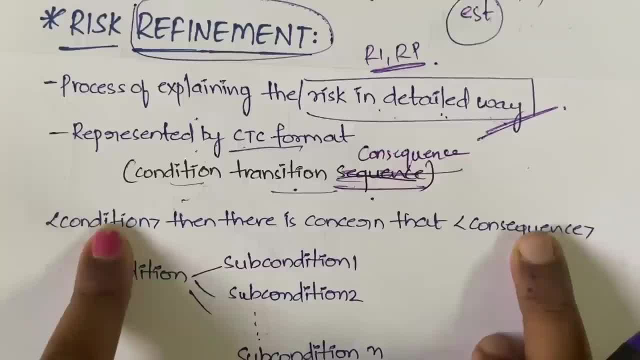 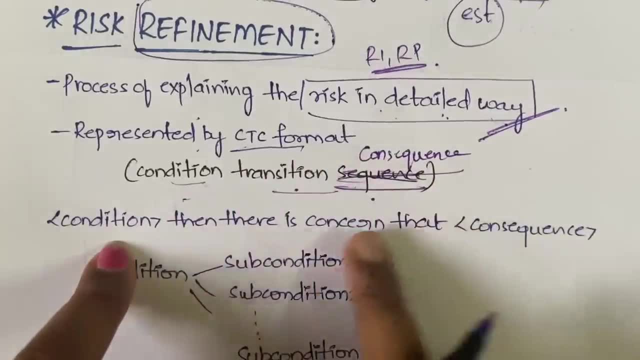 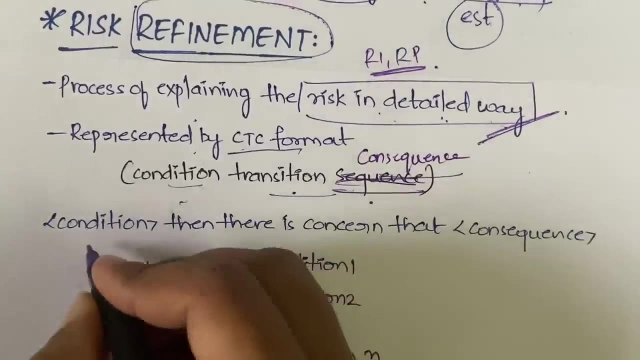 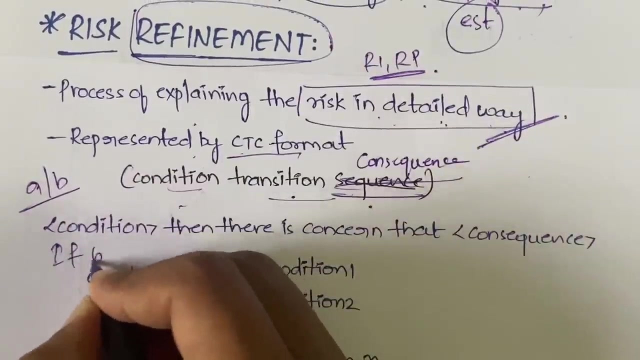 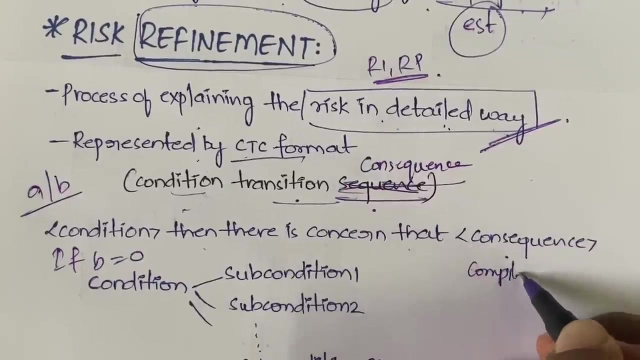 expressing in in this way: here you have condition and here you have consequence, right? if this condition happens, if this condition arises, then there is a concern that this consequence happen. ok, got it simple. if this happens, if suppose we are doing a division a by b, if b is equal to 0, then there is a concern that the compiler may throw an error because we 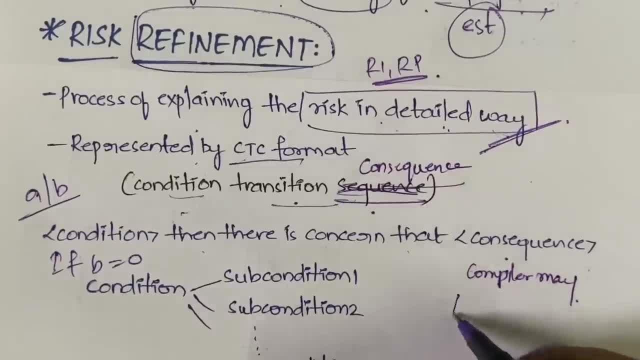 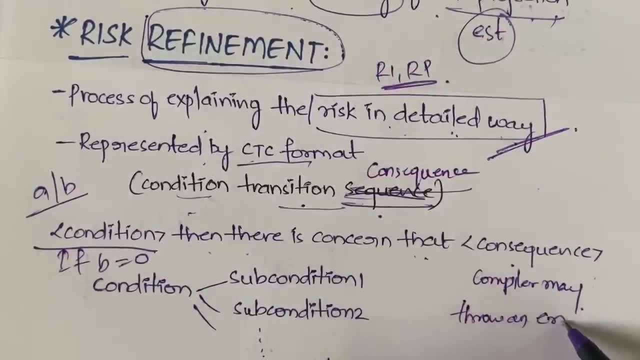 cannot divide a number with 0 right. the compiler may throw an error right, so like that. so if this condition happens, then there is a concern that this may happen. this consequence may arise. ok, this is about the risk refinement here. what we will do is we will divide a particular. 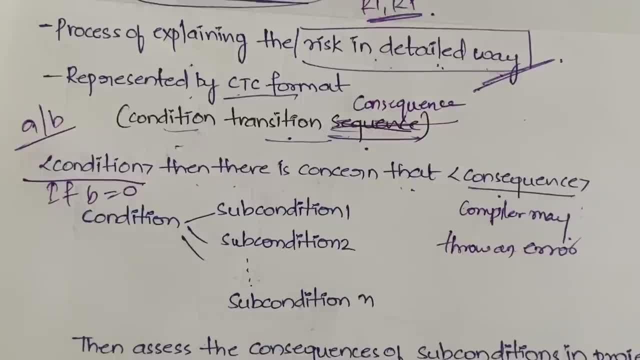 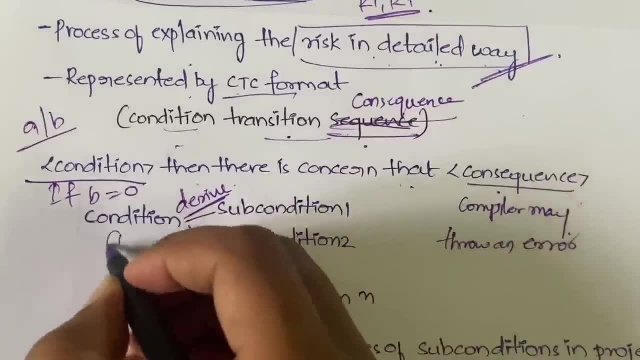 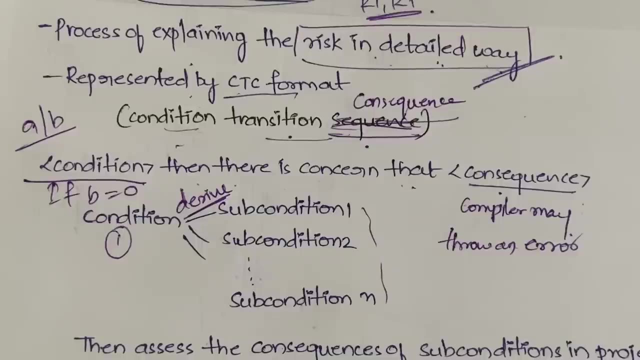 condition into number of sub conditions and after dividing it into like divide, not we say derive. we derive so many sub conditions from a single condition. ok, suppose, 1 to n condition, n sub conditions, we will be divide, deriving. then what we will do is we will divide. 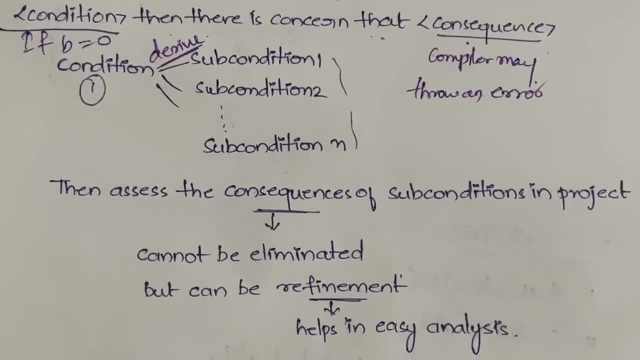 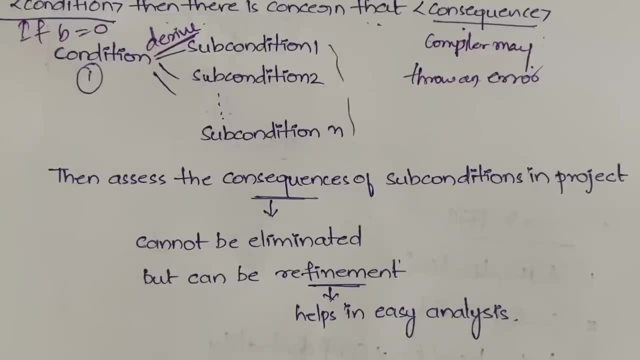 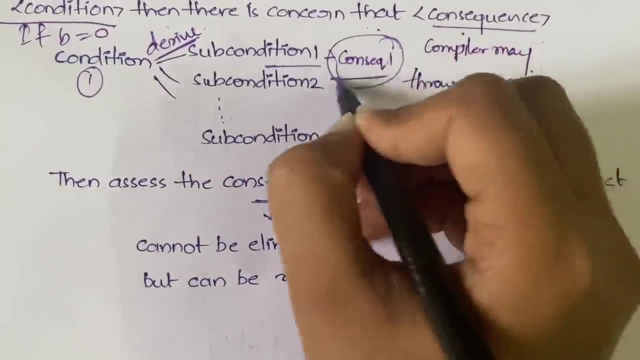 the sub conditions into sub conditions. we will be assessing the consequences of those sub conditions in the project. so each and every sub condition we will pick up and we will see the consequence of that sub condition. that is, if sub condition 1 we took and we will assess the consequence- consequence 1 we got, if this is not so strong or if that. 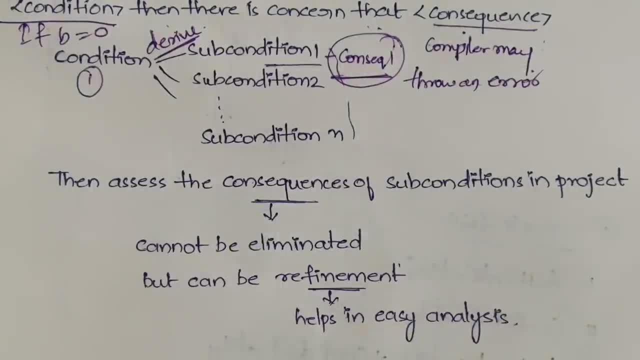 is not so important, then in that case, what we will do, we will keep it aside, which is having more consequence, which is having a lot of negative consequence. that will be the first, like that. ok, we will be dividing it into number of sub conditions and for those, 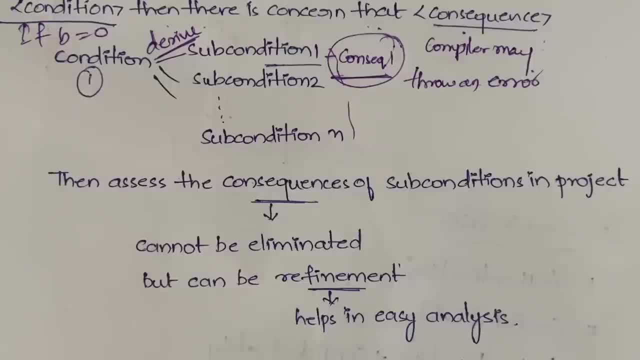 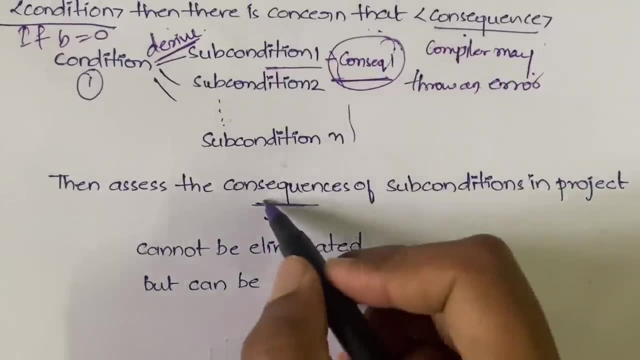 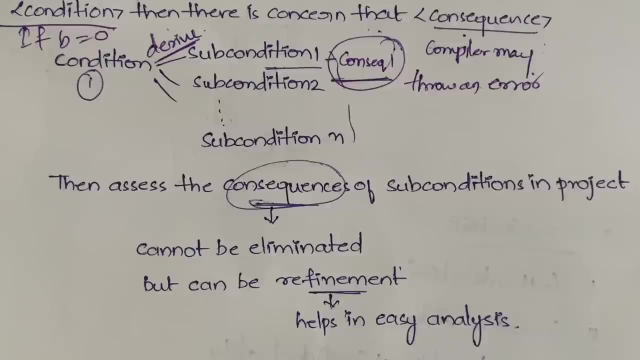 sub conditions. we will be assessing the consequences and based on those consequences then we will do the refinement. ok, so these consequences cannot be eliminated, but they can be refined. that is which is important, which is not important, which has to be given more priority. like that, you can refine and based on the refinement, you can do the analysis easily. ok, so that's. 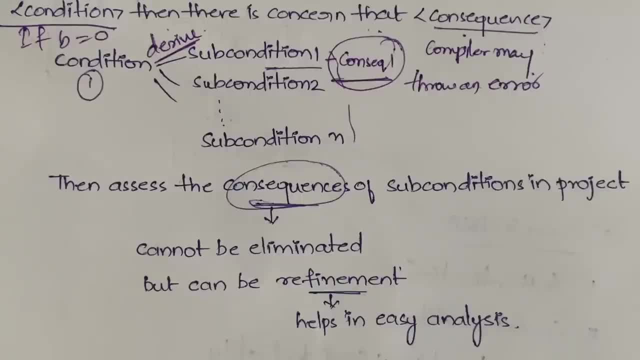 all for this video. I know by already by now. It is very important. It has become very long but still ok. in the next video I will explain about RMMM and RMMM plan also. so for this video, that's all. thanks for watching the video till the end. and if